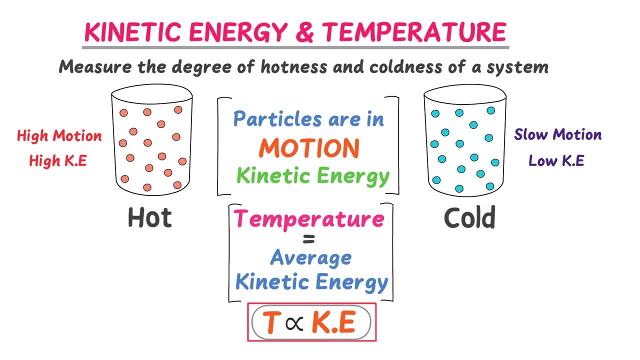 Let me repeat it: Temperature is directly proportional to kinetic energy. Now let me ask you why the temperature of this hot object is high. Your answer will be: it is because the gas particles within this cylinder possess high kinetic energy due to high motion or velocity. We know that temperature is directly proportional to kinetic energy. High kinetic energy means high kinetic energy. 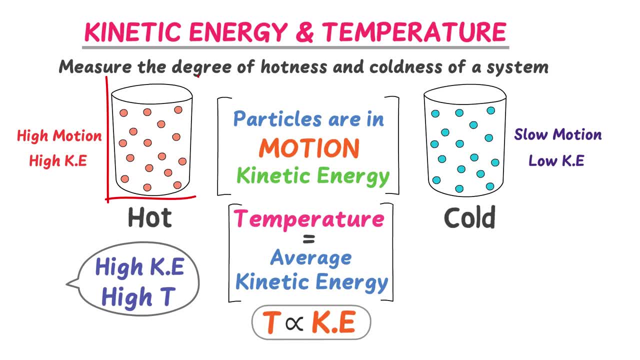 high temperature. Hence the temperature of this system is high. Secondly, if I ask you why the temperature of this cold object is low, Well, your answer will be: it is because the gas particles within this cylinder possess low kinetic energy due to slow motion or velocity. We know that. 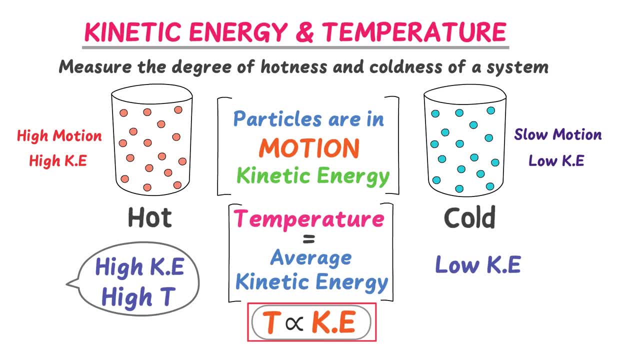 temperature is directly proportional to kinetic energy. Low kinetic energy means low temperature. Hence the temperature of this system is low and it is cold. Thus, from this example we learn that there is direct relationship between kinetic energy and temperature. Now the second important 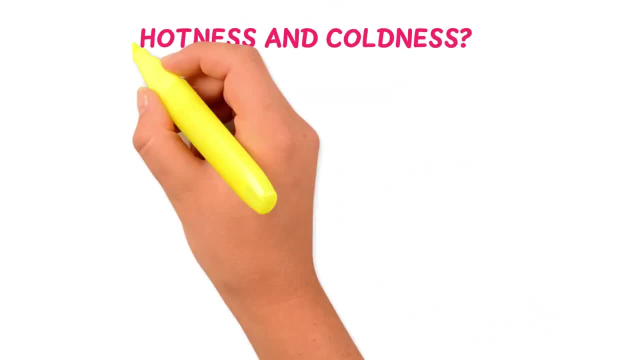 question. you should learn that- why hotness and coldness depends of any system on kinetic energy. Well, the answer is very simple. For instance, during winter season, when you rub your hands together vigorously on a cold day, what you get? Well, when you rub your hands all together, 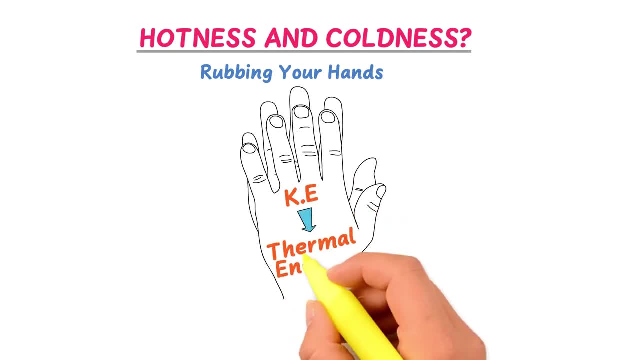 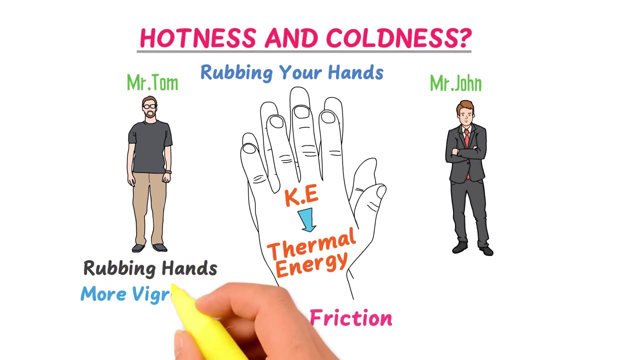 the kinetic energy of your hand is converted into thermal energy due to existence of friction between your hand. Now let me elaborate this concept further. Consider Mr Tom and Mr John. Mr Tom is rubbing his hands more vigorously, while Mr John is rubbing his hands less. 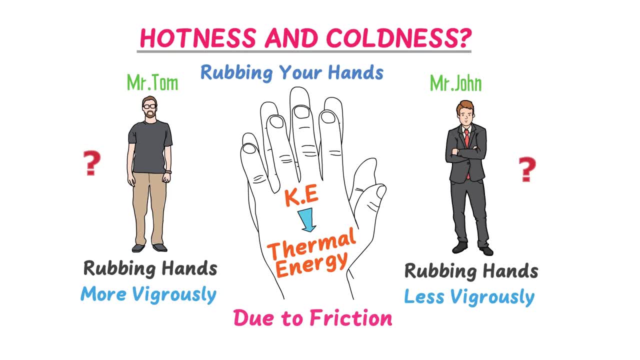 vigorously. Whose hands will get more hotness or warmth? Well, the winner is Mr Tom, because the kinetic energy of his hands is high due to high motion. High kinetic energy means more friction, and more friction means more conversion of kinetic energy into thermal. 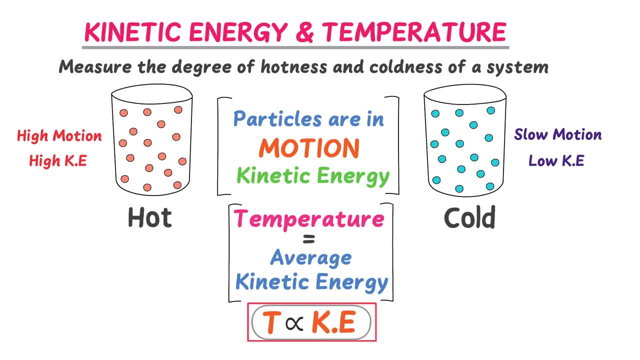 Now let me repeat it: Temperature is directly proportional to kinetic energy. Now let me ask you why the temperature of this hot object is high. Your answer will be: it is because the gas particles within this cylinder possess high kinetic energy due to high motion or velocity. 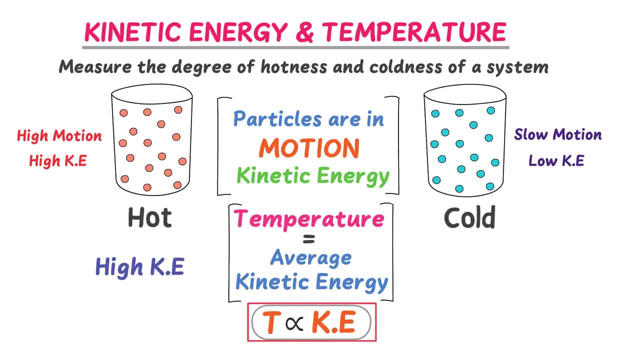 We know that temperature is directly proportional to kinetic energy. High kinetic energy means high temperature. Hence the temperature of this system is high. Secondly, if I ask you why the temperature of this cold object is low, well, your answer will be: it is because the gas particles within this cylinder. 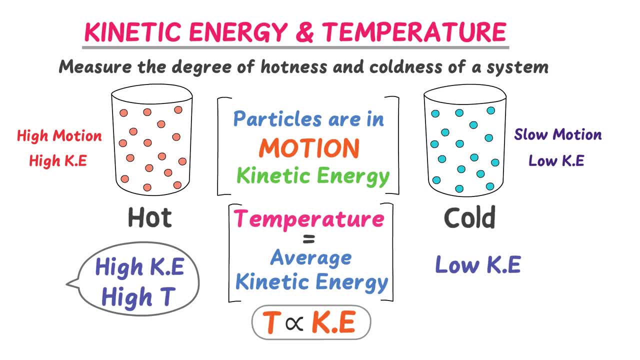 possess low kinetic energy due to slow motion or velocity. We know that temperature is directly proportional to kinetic energy. Low kinetic energy means low temperature. Hence the temperature of this system is low and it is cold. Thus, from this example, we learn that there is direct relationship between 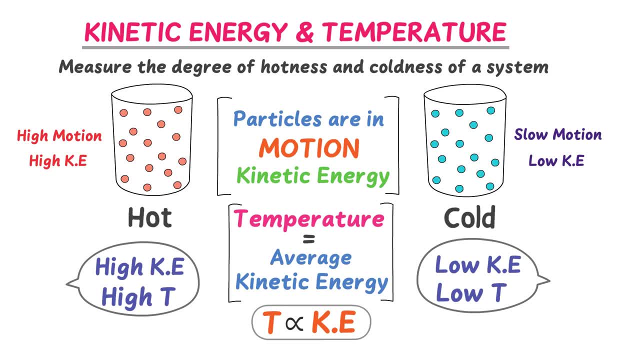 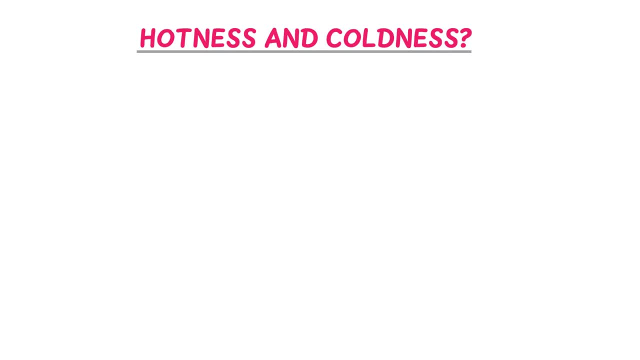 kinetic energy and temperature. Now the second important question. you should learn that. why hotness and coldness depends of any system on kinetic energy. Well, the answer is very simple. For instance, during winter season, when you rub your hands together. 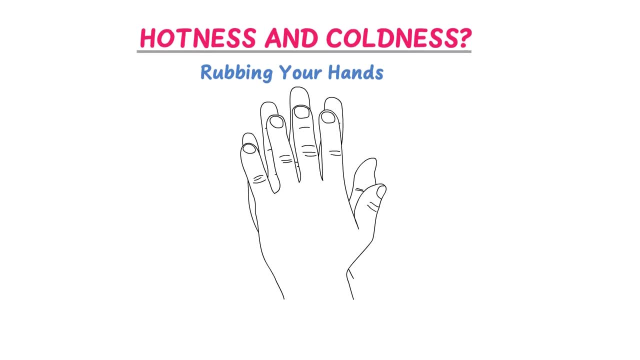 vigorously on a cold day. what you get? Well, when you rub your hands all together, the kinetic energy of your hand is converted into thermal energy due to existence of friction between your hand. Now let me elaborate this concept further. Consider Mr Tom and Mr John. 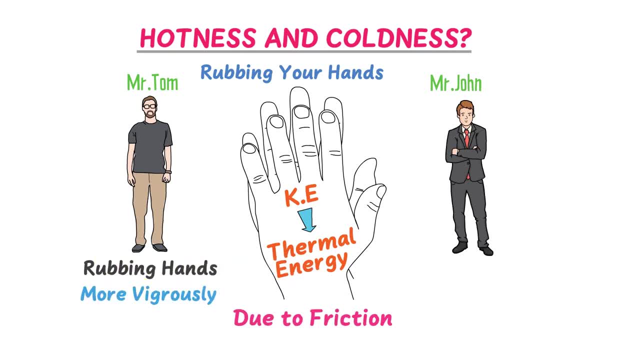 Mr Tom is rubbing his hands more vigorously, while Mr John is rubbing his hands less vigorously. Whose hands will get more hotness or warmth? Well, the winner is Mr Tom, because the kinetic energy of his hands is high due to high motion. 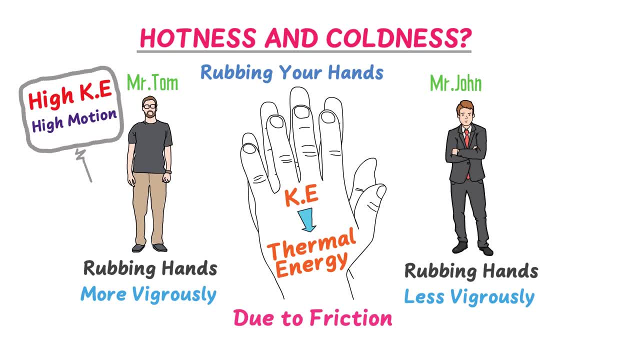 High kinetic energy means more friction, and more friction means more conversion of kinetic energy into thermal energy or heat energy, While in Mr John's case, kinetic energy of his hand is smaller due to slow motion. Smaller kinetic energy means less friction, and less friction means 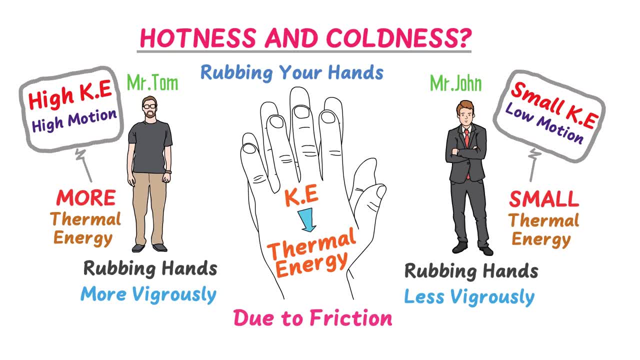 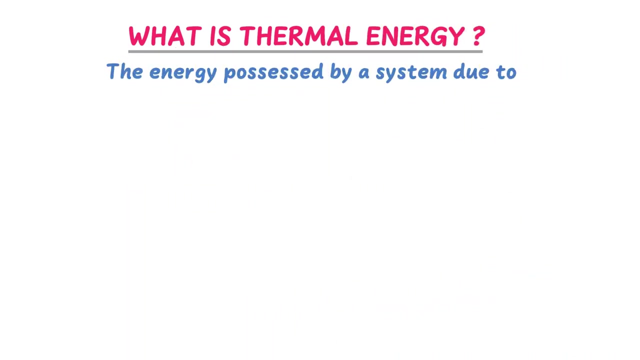 less conversion of kinetic energy into thermal energy or heat energy. You can also do this experiment right now. Therefore, remember that high kinetic energy means hotness and small kinetic energy means coldness. Now, what is thermal energy? Well, the energy possessed by an object or system due to the movement of particles or kinetic energy. 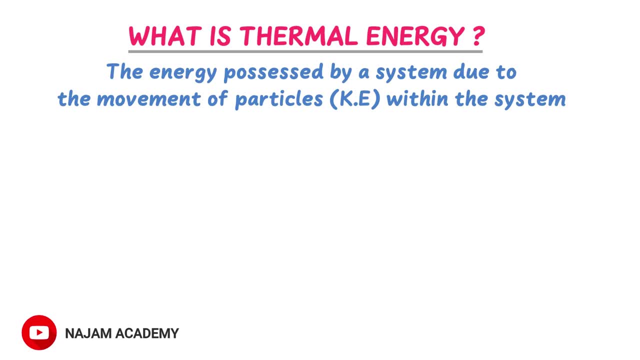 within that object or system is known as a thermal energy. For example, consider a hot object and a cold object. We know that hot object possesses large thermal energy and cold object possesses less thermal energy. If I ask you why hot object possesses high thermal energy and cold object possesses less thermal energy, 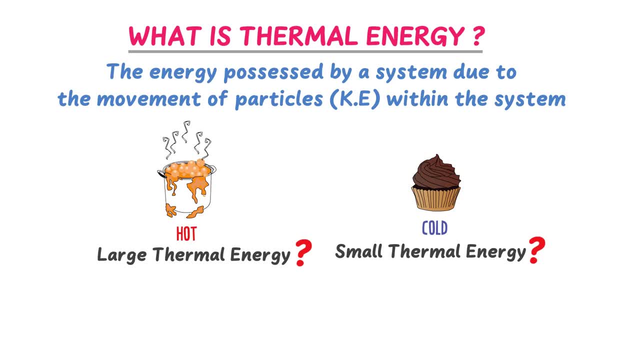 I hope you know the answer Well. the hot object possesses high thermal energy due to high kinetic energy of the particles. We also know that temperature is directly proportional to kinetic energy. Thus the temperature of this hot object is also high due to high kinetic energy. 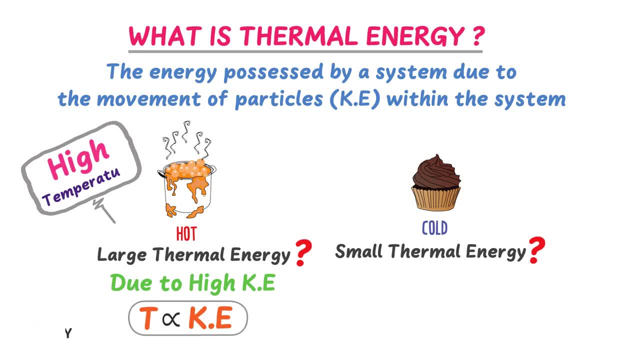 Secondly, the cold object possesses less thermal energy due to less kinetic energy of the particles. We also know that temperature is directly proportional to kinetic energy. Thus the temperature of this cold object is also low. Therefore, remember that thermal energy directly depends on kinetic energy of the particles within a system. 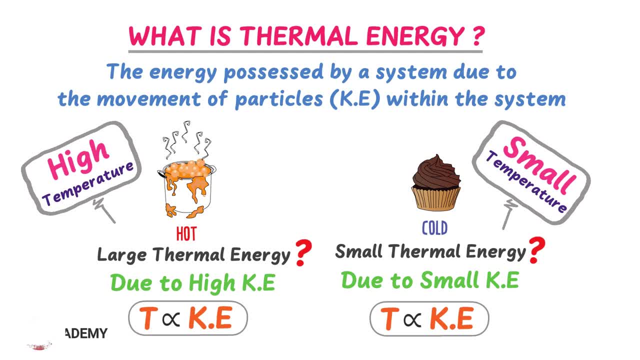 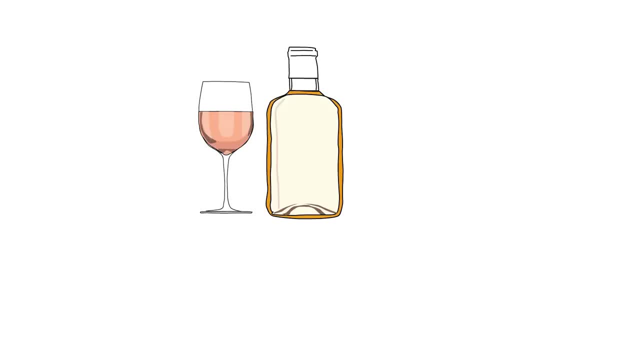 Secondly, also remember that thermal energy depends on kinetic energy of the particles within a system. Secondly, also, thermal energy depends on kinetic energy of the particles within a system. Consider a glass of water and a bottle of water at same temperature, 30 degree centigrade. 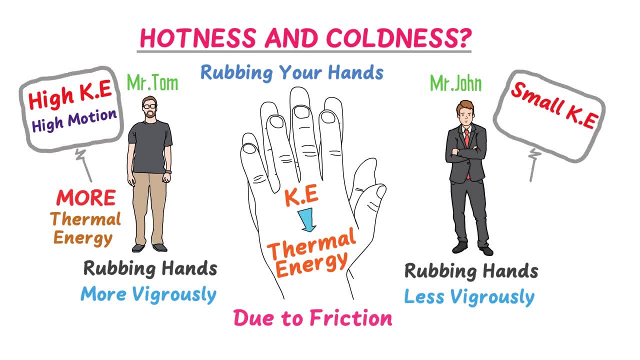 energy or heat energy, While in Mr John's case, kinetic energy of his hand is smaller due to slow motion. smaller kinetic energy means less friction, and less friction means less conversion of kinetic energy into thermal energy or heat energy. You can also do this. 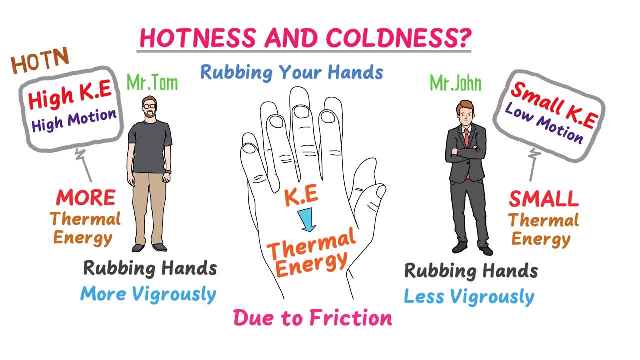 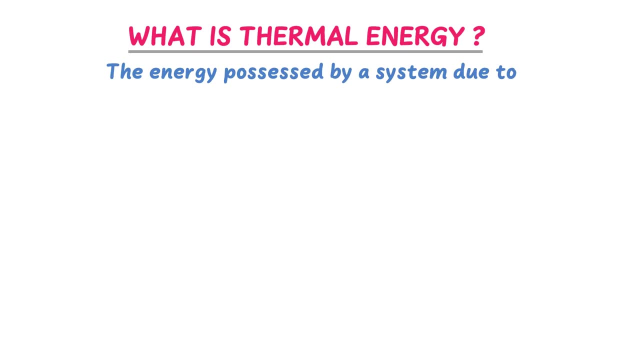 experiment right now. Therefore, remember that high kinetic energy means hotness and small kinetic energy means coldness. Now, what is thermal energy? Well, the energy possessed by an object or system due to the movement of particles or kinetic energy within that object or system is. 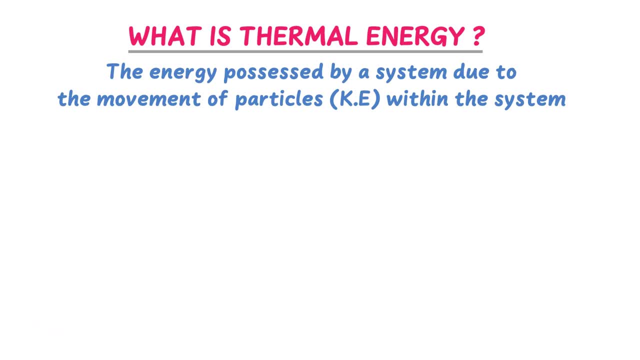 known as a thermal energy. For example, consider a hot object and a cold object. We know that hot object possesses large thermal energy and cold object possesses less thermal energy. If I ask you why hot object possesses high thermal energy and cold object possesses less thermal energy, I hope 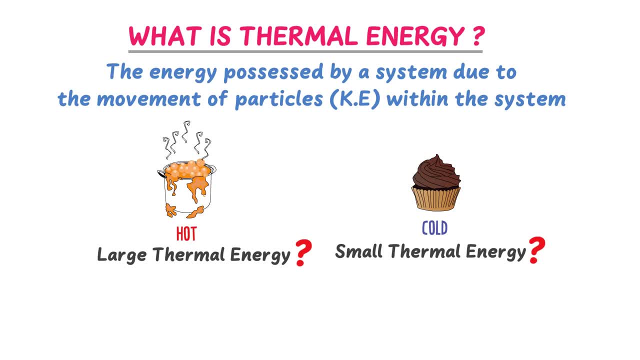 you know the answer Well. the hot object possesses high thermal energy due to high kinetic energy of the particles. We also know that temperature is directly proportional to kinetic energy. Thus the temperature of this hot object is also high due to high kinetic energy. 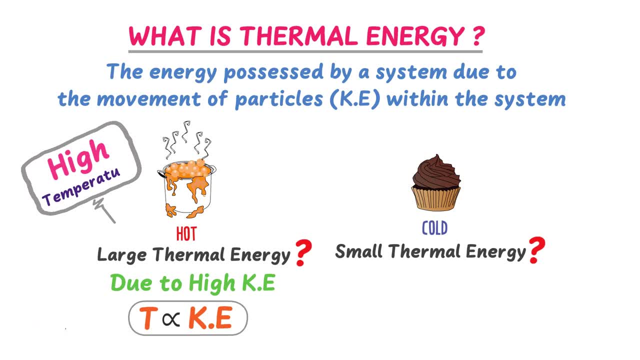 Secondly, the cold object possesses less thermal energy due to less kinetic energy of the particles. We also know that temperature is directly proportional to kinetic energy. Thus the temperature of this cold object is also low. Therefore, remember that thermal energy directly depends on kinetic energy of the particles within a system. Secondly, also remember 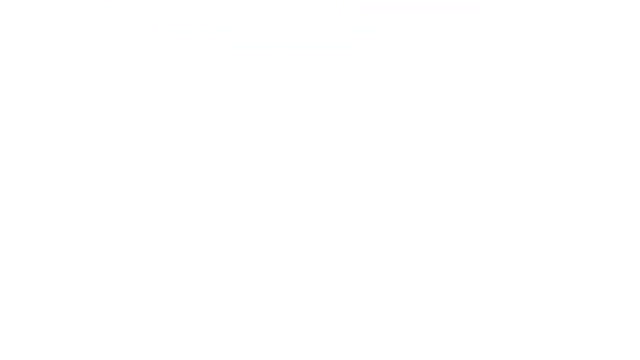 that thermal energy depends on number of particles in a system. Consider a glass of water and a bottle of water at same temperature, 30 degree centigrade. The water within the bottle possesses more thermal energy than the water and the glass, because there are more water particles in the